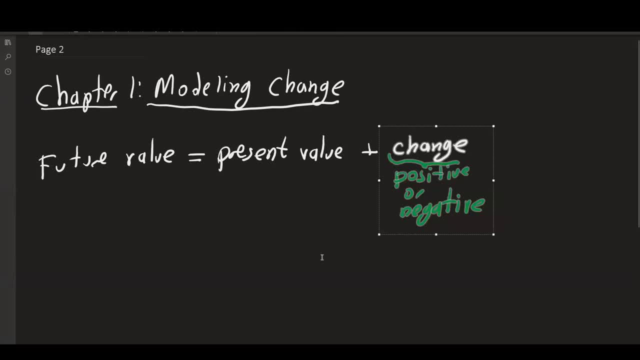 If it is positive change, then the value of that gas is going to increase. If it is negative change, then the value of the future for the future price of the gas will be less. Okay, Okay. So if you look at this equation here, 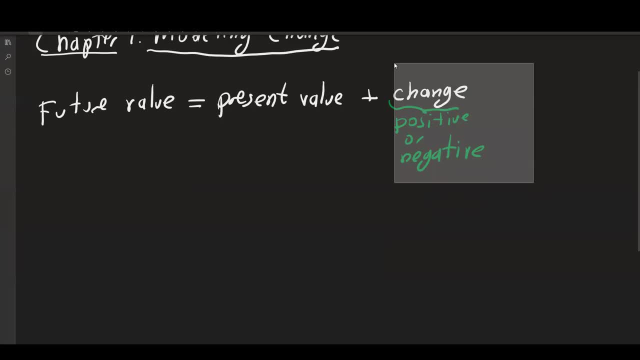 I can actually solve for change. So think about it. This is the variable. So what will be change here? So change will be equal to future value minus the present value. Okay, Okay, Okay. So change will be future value minus present value. 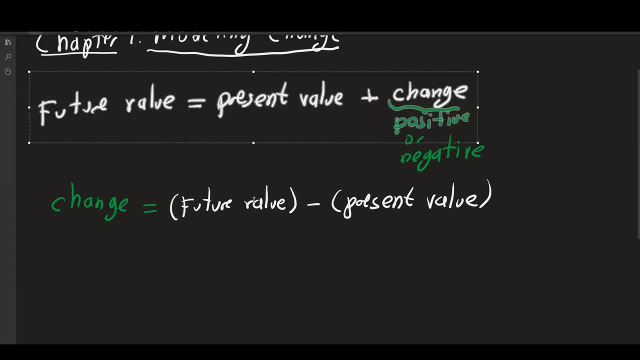 So just by looking at this, at this idea- and this is the idea that's going to be present in this chapter- The idea that future value is always present. value plus plus change. Now there is a difference between the kind of changes that we have. 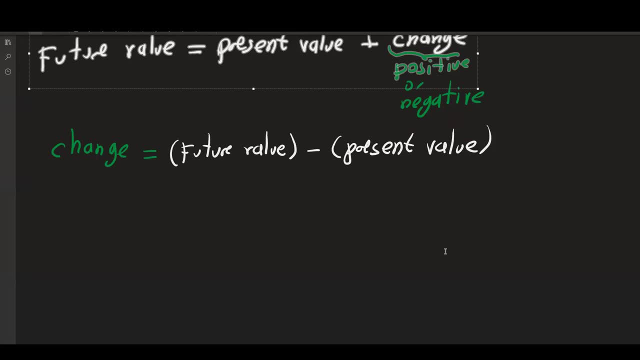 So the idea is this: So one. So if change- Okay, Okay, Okay, Okay Okay, Let's say So- change takes place over discrete time periods, then in that case we're gonna, we're gonna say that the change, then in this case change gives what we call a difference equation. 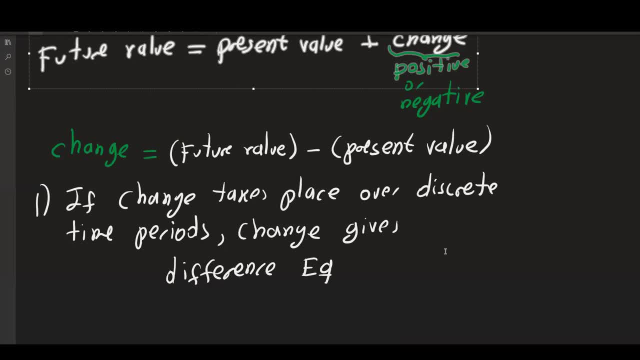 So a difference equation. So whenever change is discrete, we say we're going to get a different equation, And you will see what that is a little bit later. Now, what does discrete here mean? Discrete time periods. So these discrete time periods basically is like, for example, every day or every month. 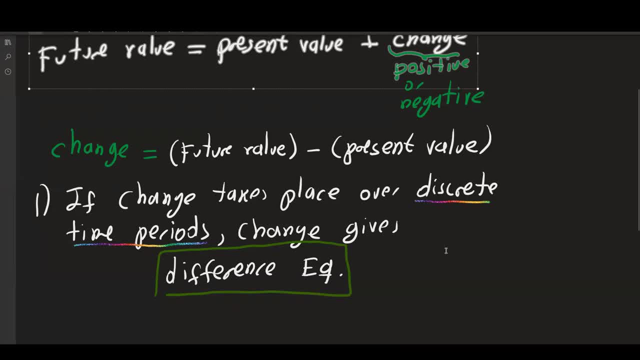 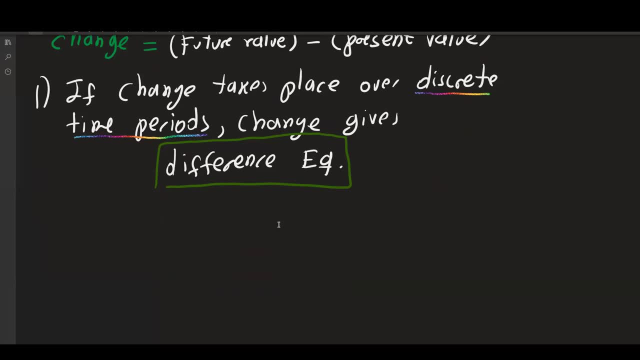 So we will consider that to be discrete, And when change happens discreetly, we're going to get a difference equation. The other way that change can happen is if it takes place continuously. So if change takes place continuously with respect to time, so continuously you can think about it, for example, as every second. 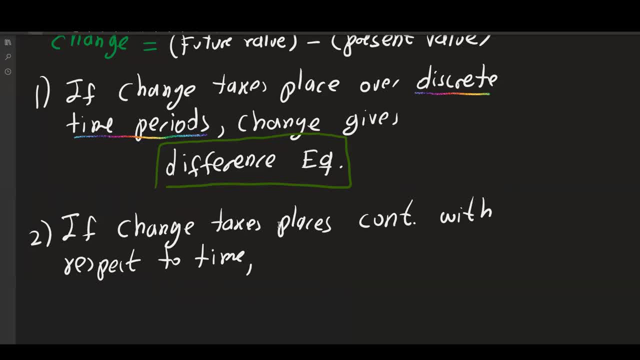 So it's always changing. It doesn't happen day by day, It doesn't happen month by month, It happens continuously. Then we get what we call a differential equation, A differential equation, And so you don't actually have to do this. 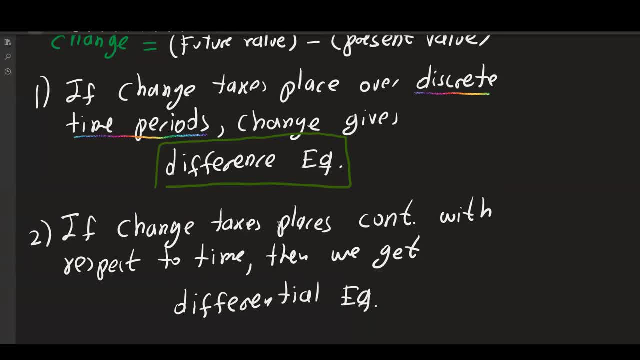 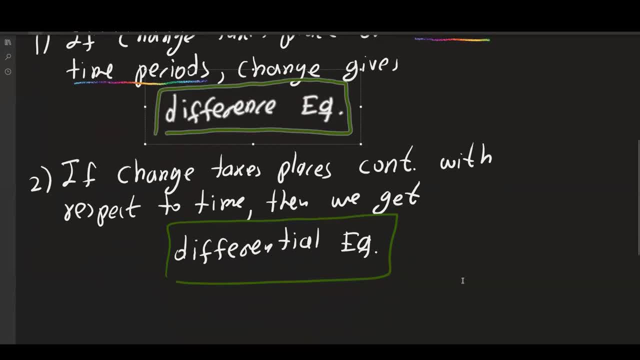 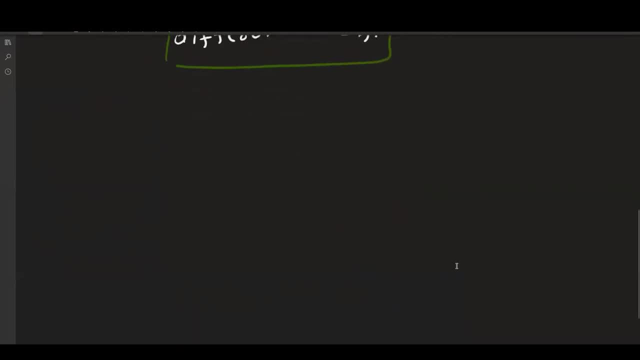 So day by day, month by month and so on. And differential equation is when change happens continuously. All right, So this is the introduction to that chapter. So I'm going to go into section 1.1, which is modeling change. 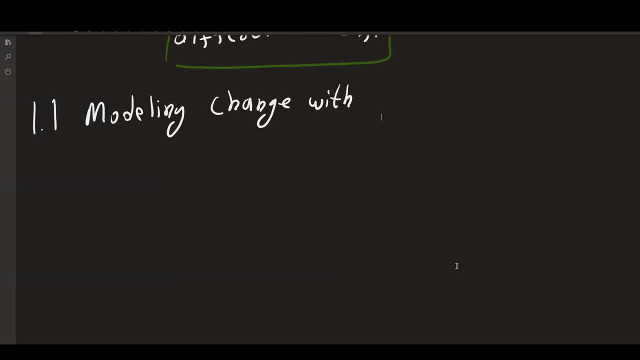 It's not really any different than any thing that's in your head. Take the different things. All right, talk to me about the different things you can do when you change. So how do you combine this with differential equation? So what do you mean, differential equation? 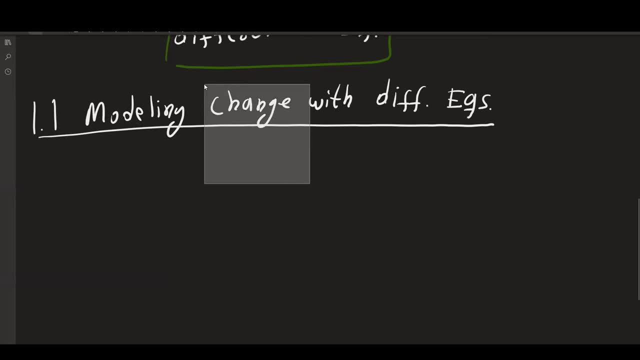 So let's go from this. So how do you do differential equation With difference equations? So what does that mean For this section? because we're talking about difference, it's not differential equation, This is difference equations- Then that means that the change is going to be discreet. 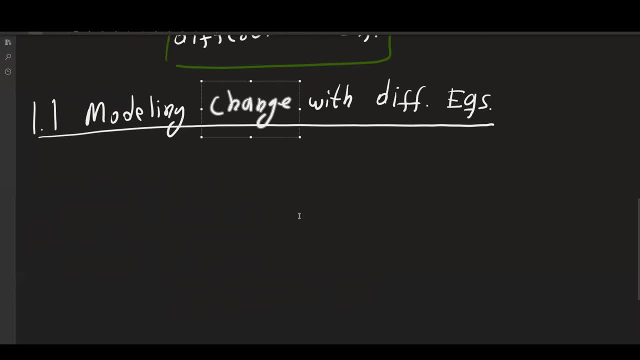 So we're going to assume that it happens every month, every day, and so on. So let me give you a definition here. So let's start with a difference definition. Okay, any questions about anything so far? Any questions? Okay, so, if A, so let's. 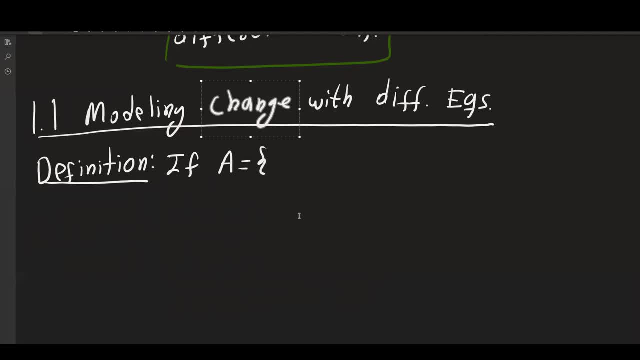 do some mathematics now. If A, so A. here is going to be a collection of numbers, for example, so A0, or a sequence A1, so here we're going to start labeling those elements of the sequence with 0, so we're going to start at 0, so A0 will be the first element in the sequence. 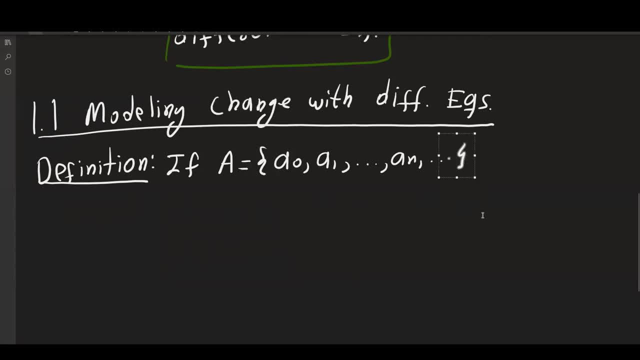 This curly braces that is here. remember this is just a notation for set, so this is a collection of a list. So if this is a sequence, so this is a sequence of numbers, so real numbers in general, then the first difference are: 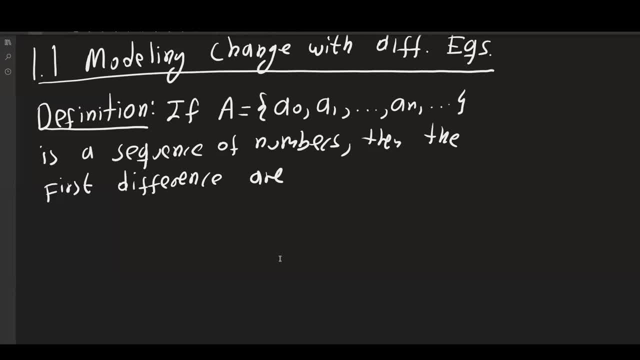 so we're going to. you will see in a second what this means. so, in terms of the picture, so we have delta. this is the capital letter. delta. delta of A0 is the first difference and is A1 minus A0, so it's basically the. 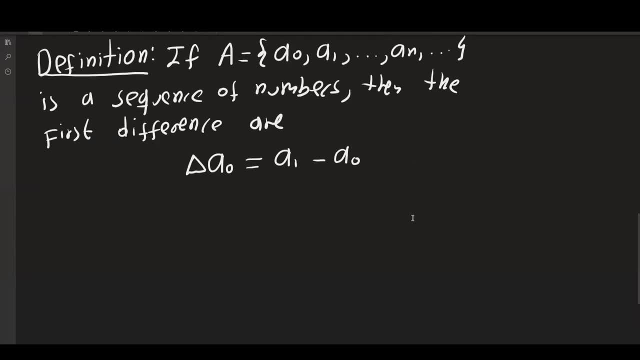 the second element of the sequence minus the first And then the next one- delta of A1, will be equal to A2 minus A1.. I will draw a picture and you will see that makes sense in a second. So let's say: 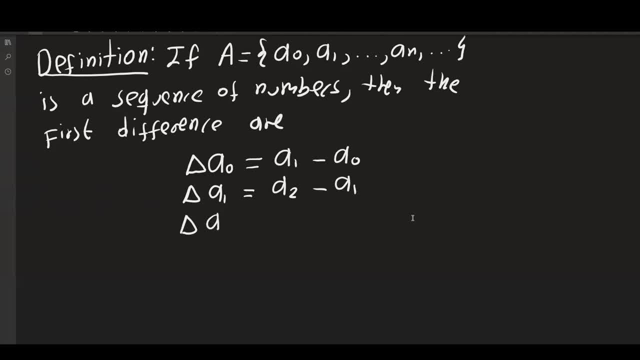 you have delta A2 and that would be A3.. Okay, minus a2 and so on, And in general what you have is a of delta of a n is equal to a of n plus 1 minus a n. So this is in general the nth difference. What 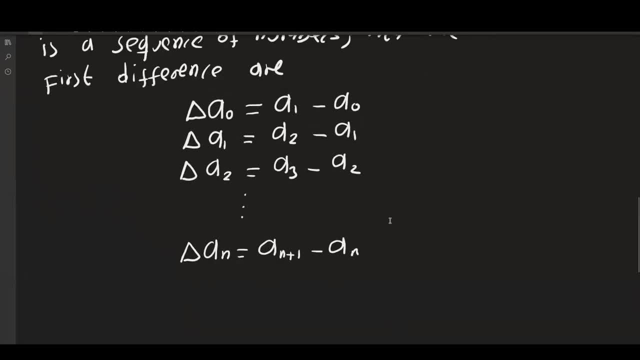 does that mean? So what is the picture of all of this? Let me draw a picture for you to show you what this actually means. So let's say, for example, you have this in the real line and your first element here is a0 and the. 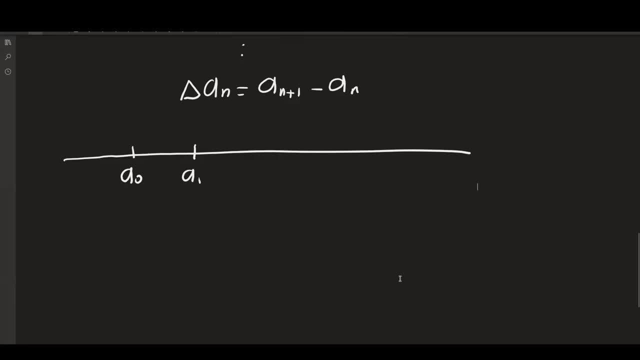 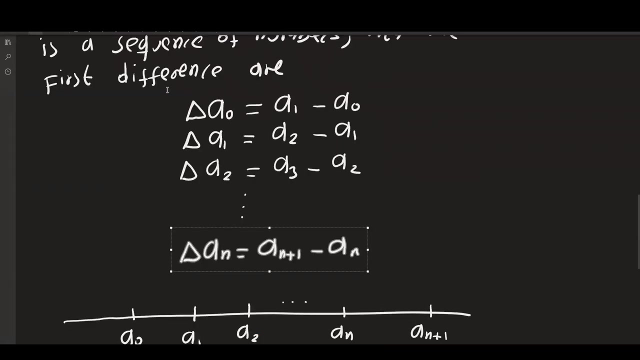 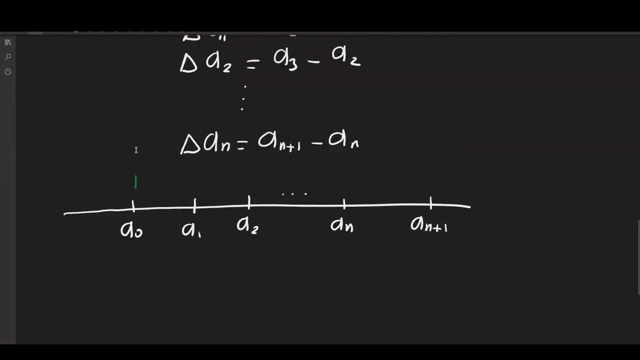 next element of that sequence is a1, and then next one is a2, and so on. Let's say all the way: later you have a n, and then you have a n plus 1.. Now, what are all these deltas that are here? The first one- this one delta of a0, is the change that happens in the 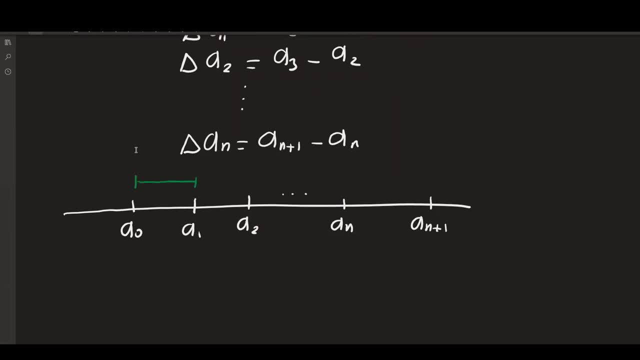 first part from a0 to a1. So this is a of delta of a0,, okay, And the next one is a1. Is that change? whatever the distance between a1 and a2 is, So it's going to be delta of a1 and so on. So this one is the last one. This is delta of a n. So 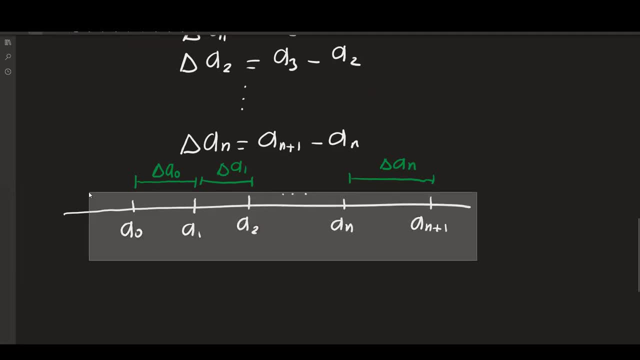 this is actually the distance. If you look at this as a sequence of numbers, in the real line, the delta corresponds to the distance between the delta. a0, corresponds to the distance between a0 and a1. and so on, for all of those things. 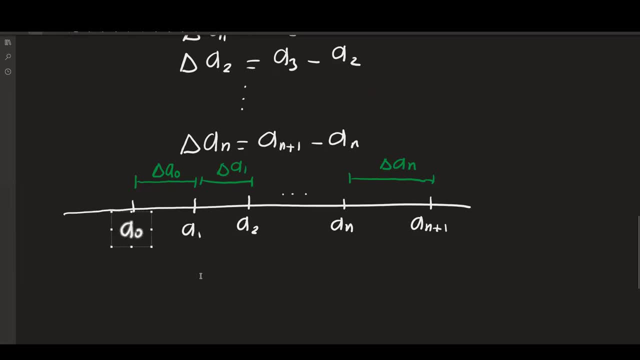 So that way is the difference. So, when you have the distance between a zero and a one, that is, a one minus a zero, and so on for the other ones. Okay, is that clear for everybody? Yeah, Okay, any questions? Okay, any questions about any of that? 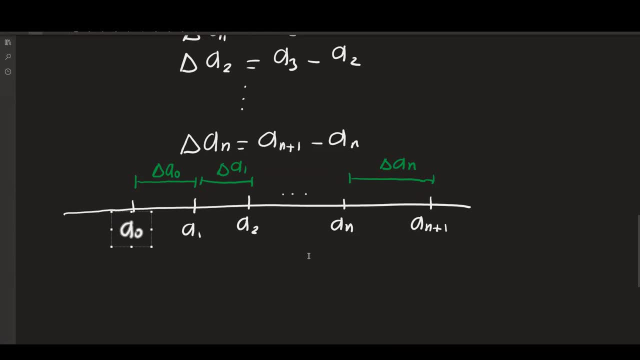 Now why are we talking about this here? Because imagine that this a n here the a n is the present value and a n plus one is the future value. So the future value will be equal to the present value plus whatever the change happens in that interval. 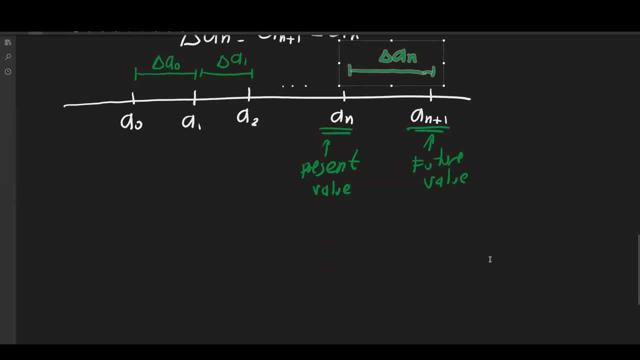 Okay. is that making sense for everybody? Is that clear? Yes, Okay. so if you write down, a n plus one equals a n plus delta of a n. we are saying that the future value. we are saying exactly the same thing we were saying before. 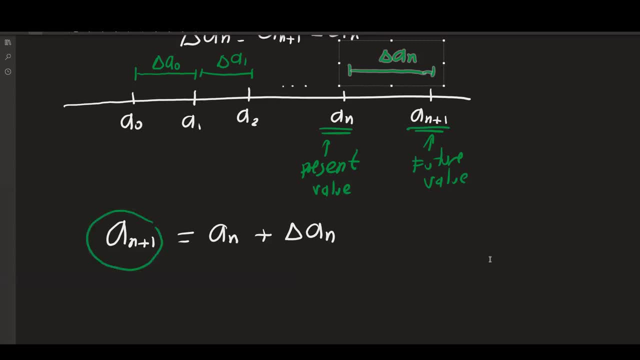 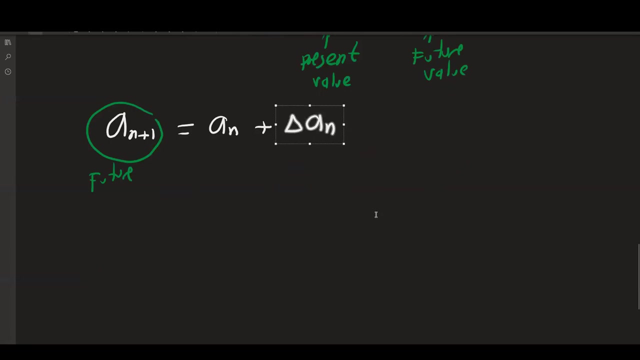 We are saying this is the future value is equal. okay again. so trying to update, give it a second. So this one is the present value plus whatever change happens. so delta of a- n is just a fancy way to say that's just. 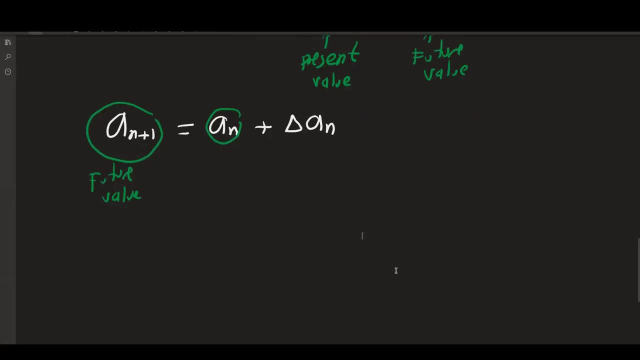 the change. The idea for what we're gonna do later, actually in this section, is because we want a formula for the future value. we're gonna know what the present value is and basically what we want is to find a formula for the change. 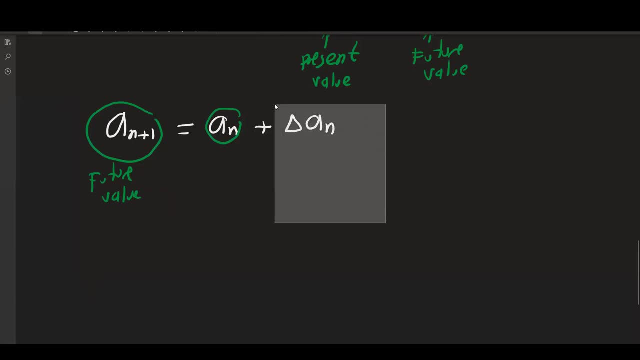 So once you figure out the change- and you, of course, know the present value- then you can figure out what the future value will be. okay, Okay, so all right, so let's actually do so. this is all like a preparation for it. 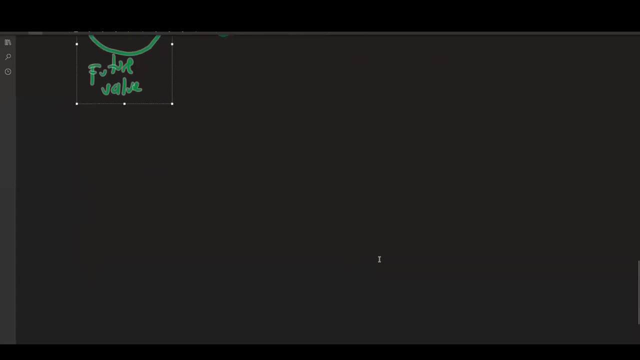 So let's do actually an example, So some example here. So let me give you an example, So an example of a savings certificate. So let me say what that, what the example is. So let's look at the initial, So the initial value. 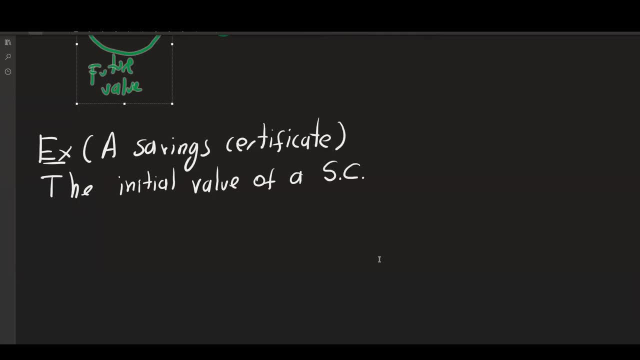 of a savings certificate. I'm just gonna say SC is, let's say, $10,000.. So we have a savings certificate. So that's basically the initial amount of money that you have in that savings certificate. So this savings certificate accumulates. 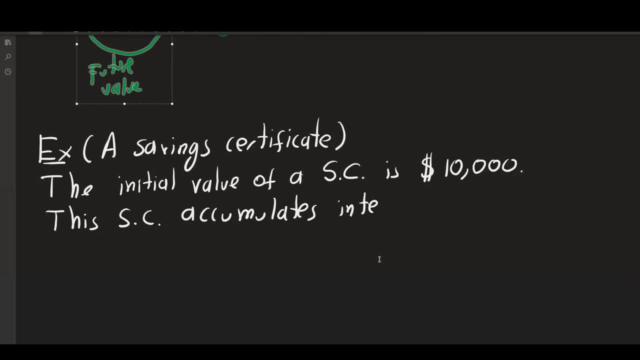 so that accumulates interest at, let's say, 1% per month. So every month you get 1% of whatever you had in the account. All right, so what happens in this particular case? So when you start? so let's look at a picture here. 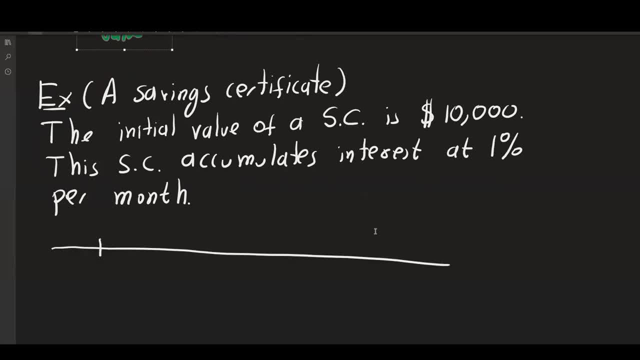 Let's look at a picture. So when you start, you start, let's say, with $10,000.. $10,000, okay, That would be your A0, right? So your initial investment on that savings certificate, So that would be your A0. 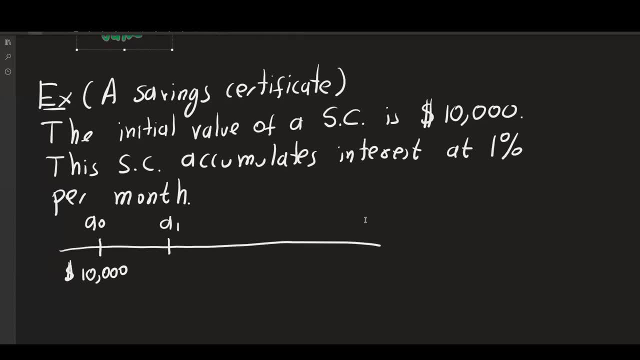 Now A1, that would be at the end of the first month. that would be the amount of money that you have, applying this 1% and so on. So you have, for example, A2, that would be the money that you have. 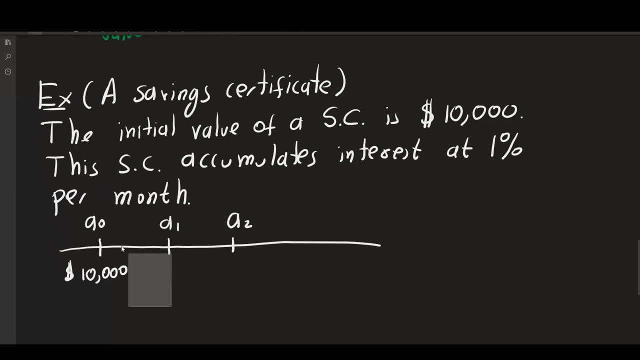 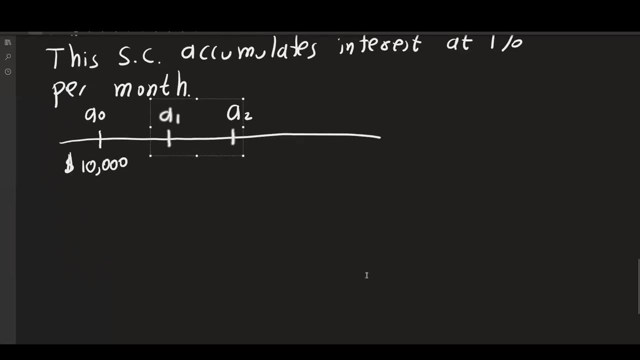 at the end of the second month. So this here is the first one, this here is the second month, and so on. okay, So making sense. Any questions about this? Any questions? All right, so then let's say A. 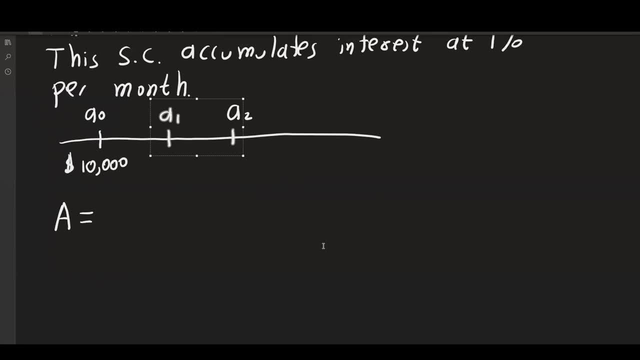 So I'm gonna give you the sequence here and I'll explain where how I got this the sequence. So let's say 10,000, this is gonna be your A0.. So this is gonna be the initial, the initial amount. 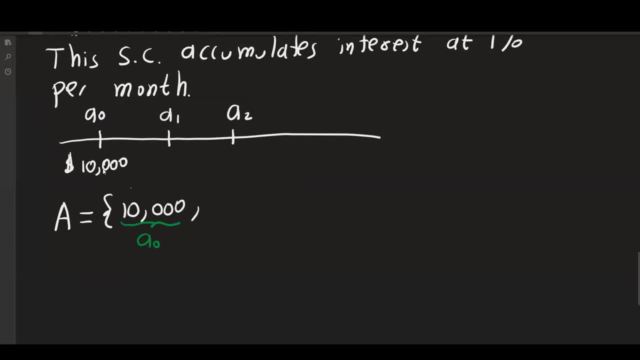 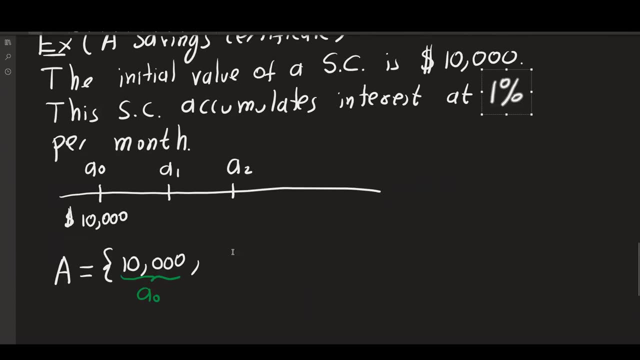 So that's gonna be the A0.. Now, that's the one that is here. Now you're gonna apply a 1% on it, So that means the next, the A1, which is gonna be this value right here- is gonna be $10,000 plus the 1% that you make over that: 10,000. 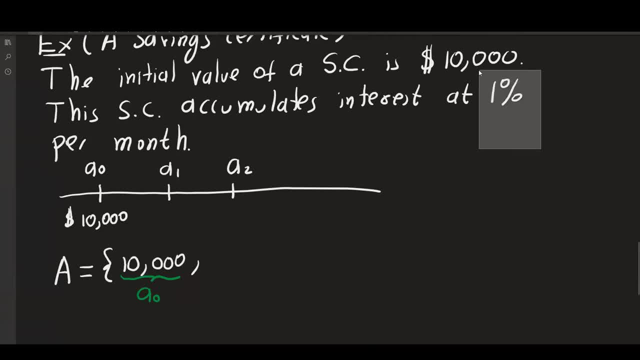 Now, if you actually use a calculator, 1% of 10,000 will be $800.. So at the end of the first month you will have 10,100,, all right? Okay, That would be the value of A of A1. 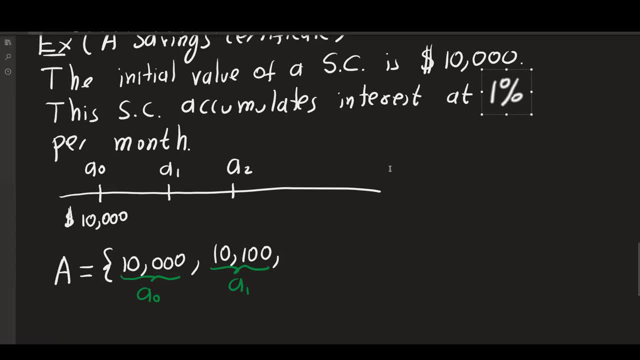 All right, so now what happens for the next one, which is gonna be the A2?? So this one is A2.. Now this 1%. so let me ask you a question here: Is this 1% for this value of A2?? 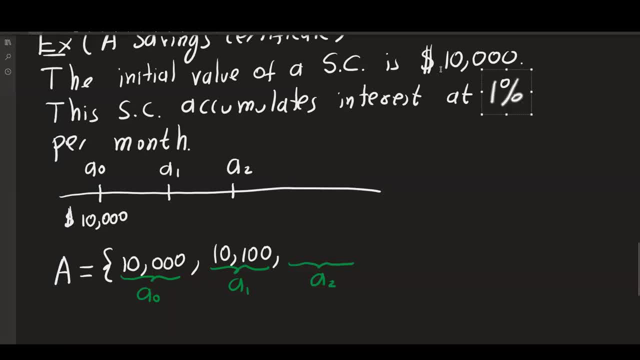 Is this 1%, a 1% of 10,000? again, Exactly the 10,100.. So I'm gonna take 1% of this and then I'm gonna add it to this one again, right? So that's gonna give us. let's say what's it gonna say? 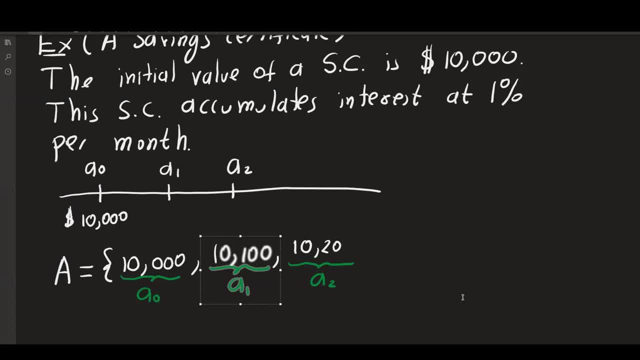 It's 10,200.. And one. if you compute that and you continue that way, the next one will be 10,303, and that will be the value. this is gonna be the value of A3, and so on. right. 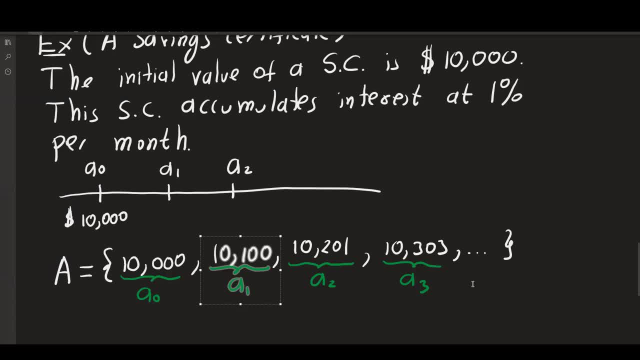 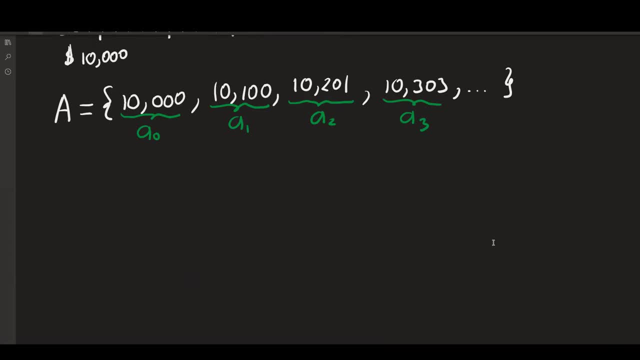 And so on. so you will have a sequence there of those values, okay, So let's recap again. So what is A0?? So A0, here it is, Here it is Here it is Here is the initial value. 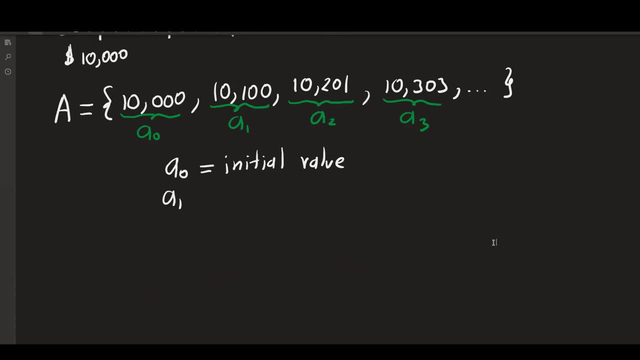 So this is the initial value. A1 is the value at the end of the first month, and so on. A2 will be the value at the end of the second month, and so on, and so on, So on and so forth. right, 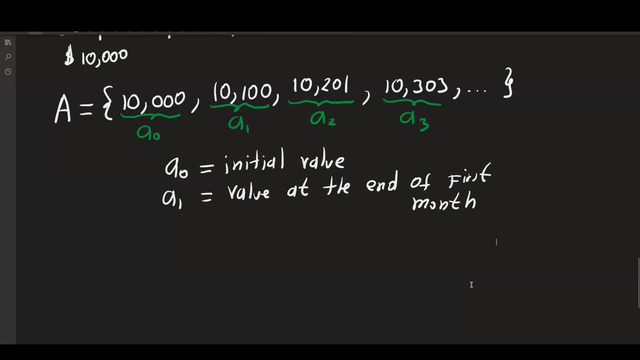 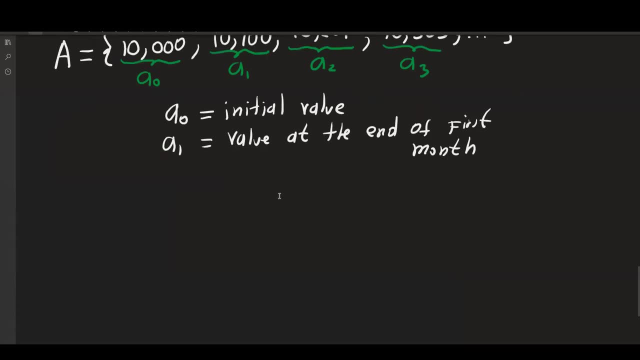 All right. So let's try to actually get some kind of formula for this, and this is where the difference equation is gonna come into play. Now, remember what the model we have, which is this: The future value, which is an plus one. 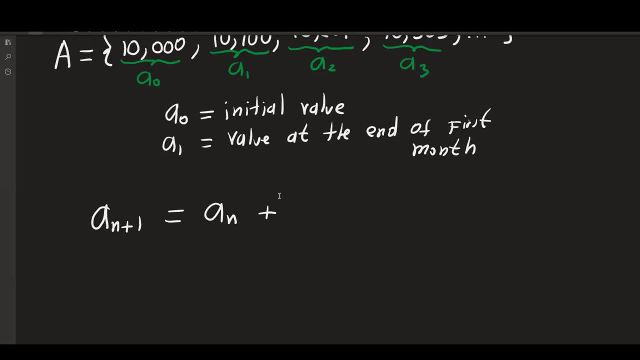 is gonna be equal to an plus delta of an. So in most cases, what we want is to have a formula for delta of a- n. So that's what we want. So most cases, we want a formula for this. So we want a formula in terms of a- n. 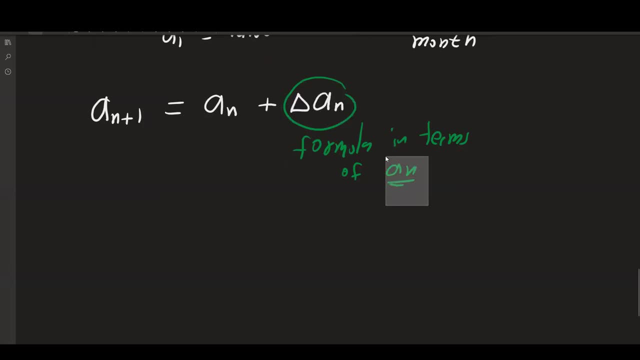 Why? of a n? Because that is the present. So we're supposed to know this. So once we get a formula for this in terms of a n, the right-hand side of this equation will be all in terms of a n, which is the present. 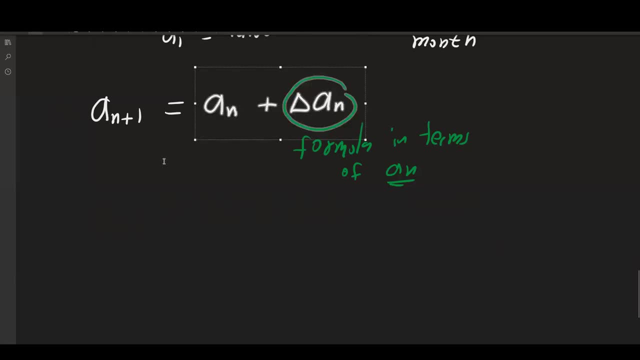 So that way, knowing the present, we'll be able to predict what happens in the future. So let's try to get a formula for this, for this delta of a n. Now, to get a formula for delta of a n, let me draw again the picture here. 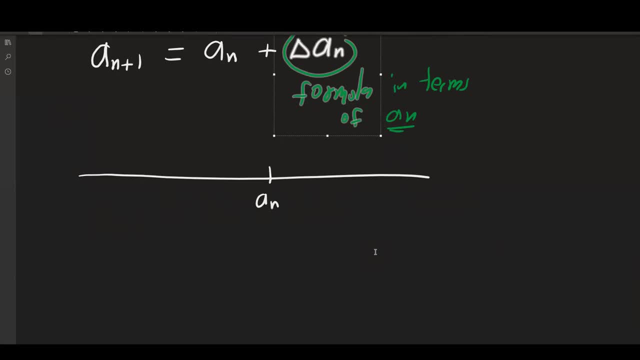 So let's look at what happens in the formula. So this is a n, that's the present, And then we have a n plus 1, that is the future. And this delta of a n is the change that happens between the present and the future. 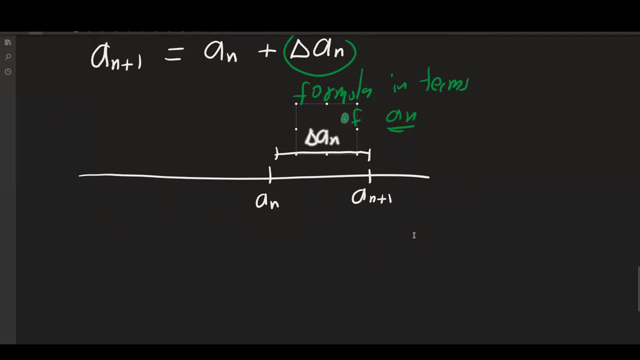 So we want a formula of what happens here. So what is this delta of a, n Now? so let me ask you a question In this, in this month, in this month, right here this month: what changes there? What is the thing that changes in general? 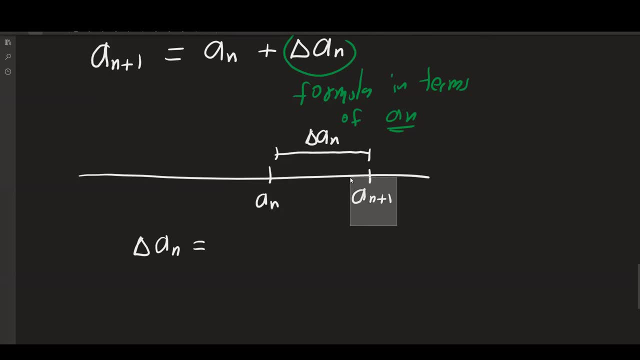 You start with an amount. How do you get to the next amount? What is the thing that changes? makes the change there? The interest right, Exactly. So this is going to be the interest, The interest paid. Okay, And dollars. 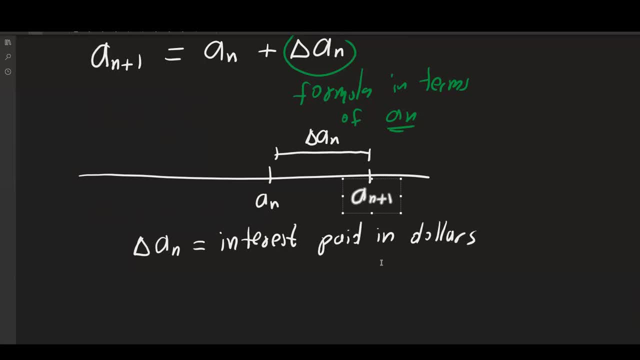 So that's what changes there Now, because we are looking at this month here. this is the interest pays in dollars. That's the interest that we are getting. That's the 1%. Now. this is 1% because we are looking at this delta of a n. 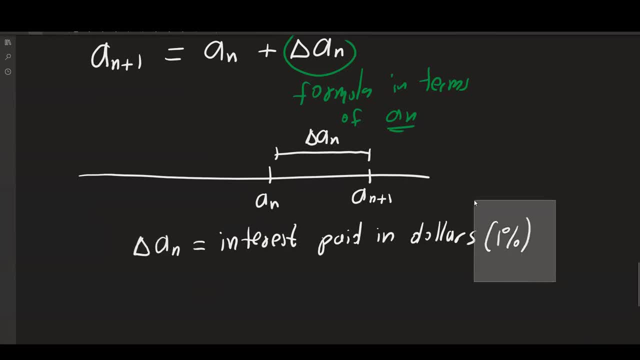 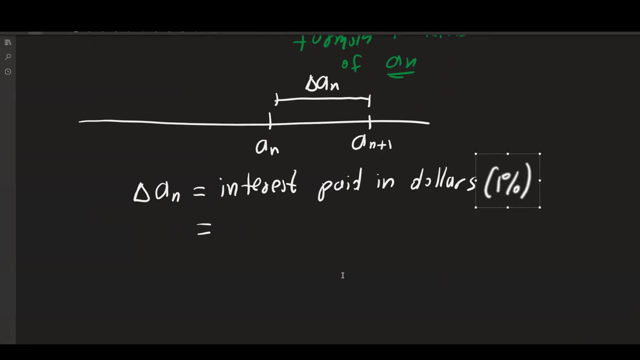 Let me ask you this question: This is 1%? of what quantity Exactly? So this pretty good. So this is going to be equal to 1% of a n. All right, So what is 1% of a n? 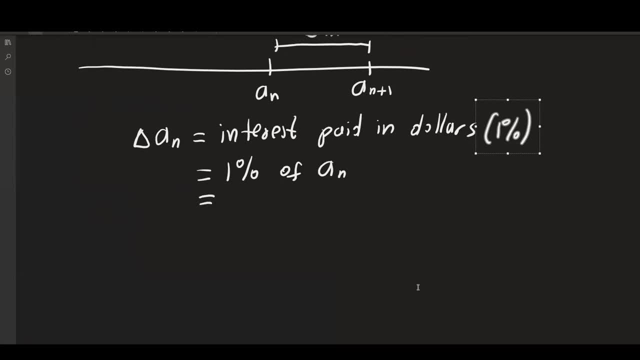 So just basically multiply by 0.01, right? So let's translate this mathematically. So it's going to be 0.01 that multiplies a n, And this is one of the things that we wanted to do. So we wanted to get. 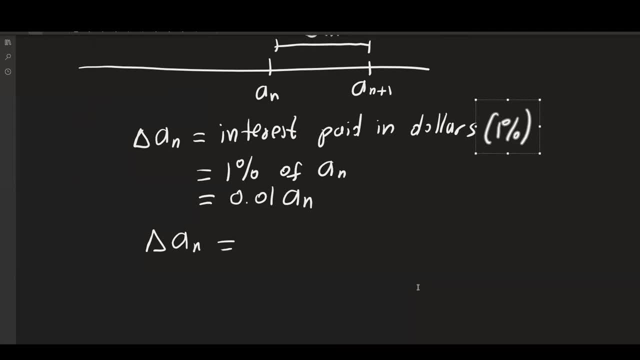 A formula for a n, for delta of a n in terms of a n. Let me correct this here. So this is what we want: We want a formula for delta of a n in terms of a n. Okay, So let's go back to our formula here for the initial formula. 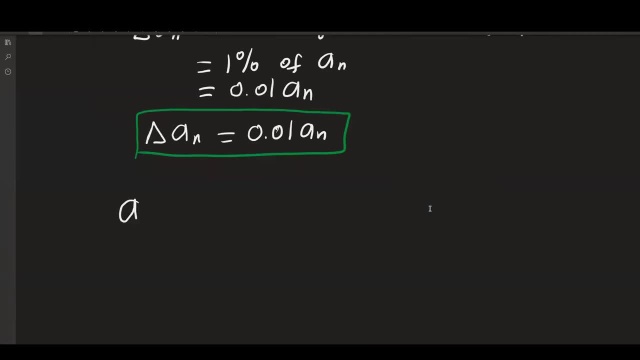 Which is what we always are doing in this section. So a n plus 1,, which is the future value, is going to be the present value, a n plus this delta x. But what is this delta x? This delta x is this quantity: 0.01 a n. 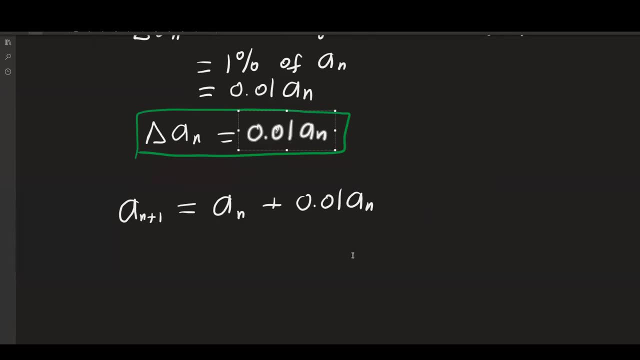 Okay, All right. So Let's simplify this formula here. So let's look at this. So these are like terms, So we can actually write down what is a n plus 1.. So a n plus 1 is equal to: 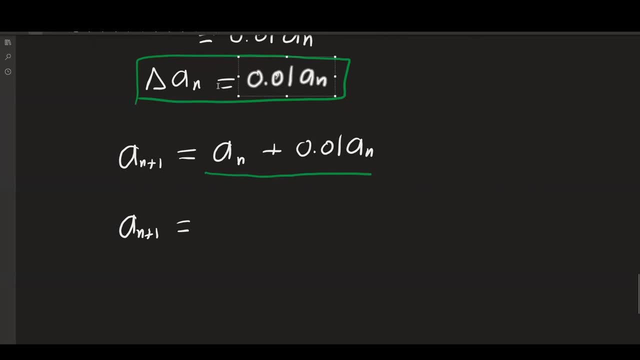 This is basically what we have here is 1 times a n plus 0.01 a n, So that's going to give us 1.01 a n. Okay, So This is the formula we were looking for, So we can predict the future. that's a n plus 1, in terms of the present, with this formula. 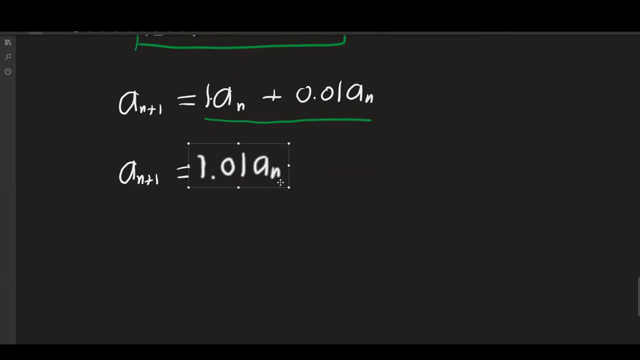 that we have here. So remember this: a n represents the amount of money that you have in that saving certificate. Now there is something missing here. This is what we call a recurrence formula. All right, A recurrence formula. basically, what that means is it's calling itself. 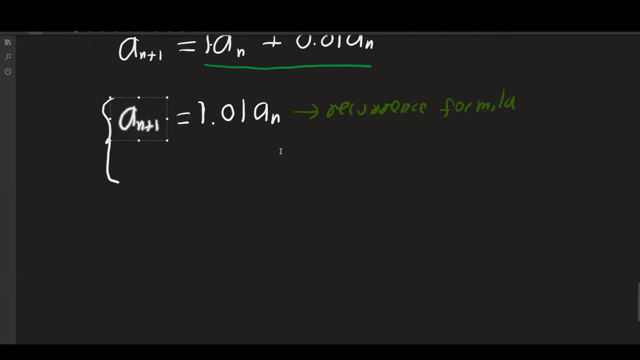 So it's a sequence of the a n's or a n plus 1, in terms of the previous one. So this is a recurrence formula And there's something missing, which is the initial condition. So the initial condition is a 0.. 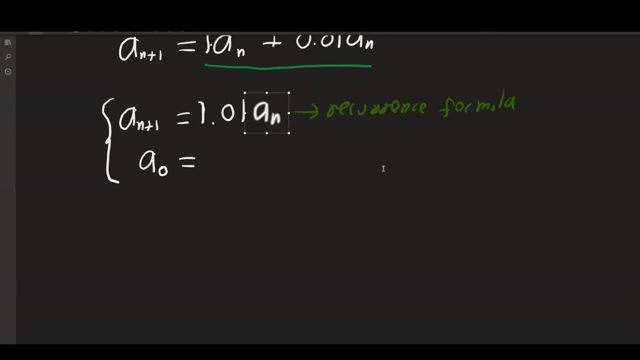 So the starting point of your sequence. So you have a sequence: a 0, a 1,, a 2, and so on. You have a formula To construct the whole sequence, which is this one, But you also have to say what is the initial value of a 0. 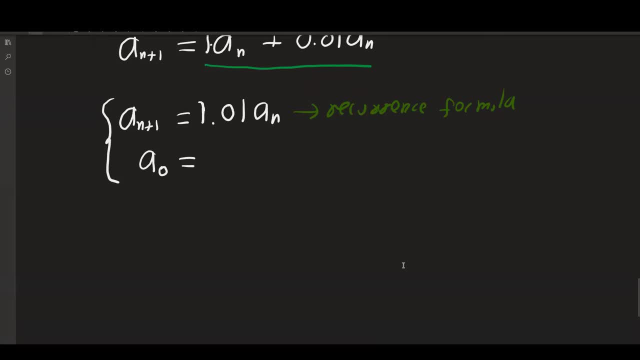 Now, what is? So? let me ask you a question here. What is a 0 here? So that's the 10,000.. So this thing that is here, both of these things together, is what we call a dynamical system. 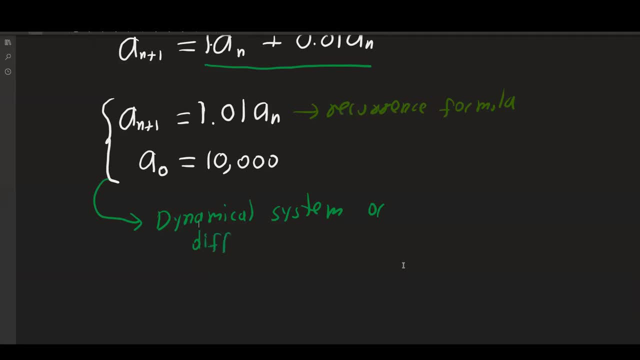 Or difference equation, So when you're looking at this type of things. so this is where this section 1.1 is usually about. It's about you're going to come up with some kind of recurrence formula for the sequence. We have this discreetly. 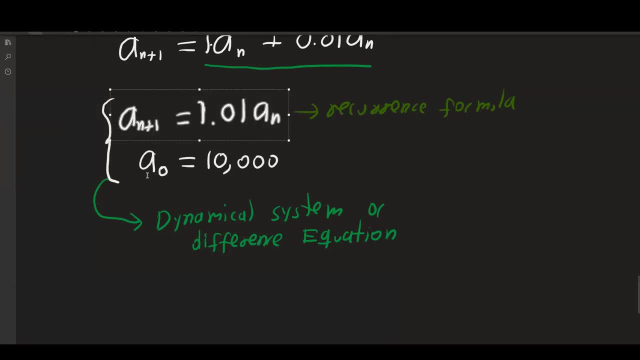 This happens every month, And this is the initial condition. So that's why we call it difference equation, Because it happens discreetly. Okay, All right, So I'm going to show you now. So what do you do with this type of formulas here? 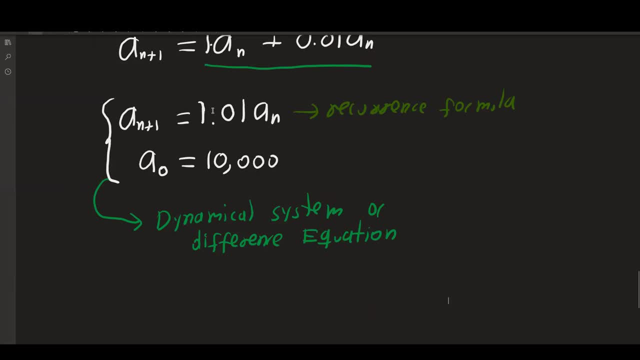 Now you can put this, maybe in Excel and do it. What we're going to do in this class is use Mathematica for this type of computation, So I'm going to show you how we can set up this type of difference equation in Mathematica. 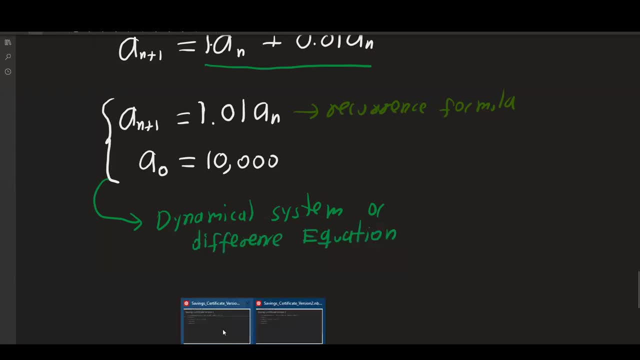 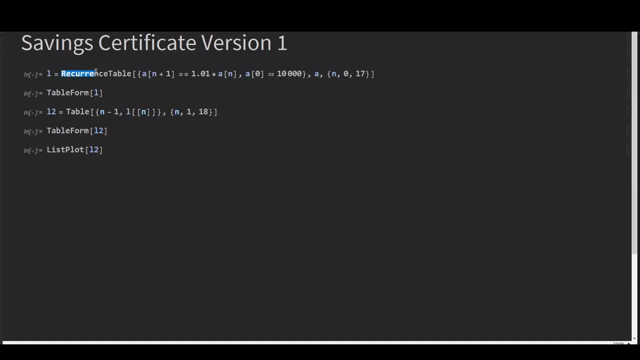 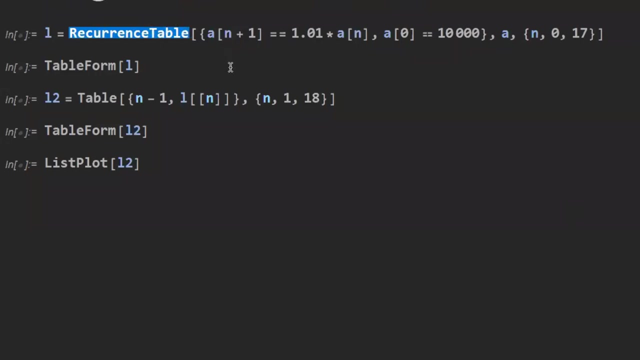 to give us some values. So I'm going to show you here in Mathematica. Okay, So the code for Mathematica to work for difference equation is this one that is here. It's called recurrence table. If you start typing recurrence, it's going to show up one of the things that you can. 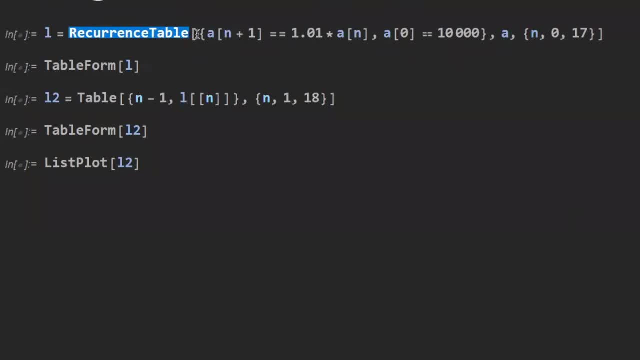 do Now? what is the syntax for recurrence table? So it's always open bracket, close bracket, here. And here I'm going to put my formula. You see, this is the formula. I had right, This is a n plus 1 in Mathematica. 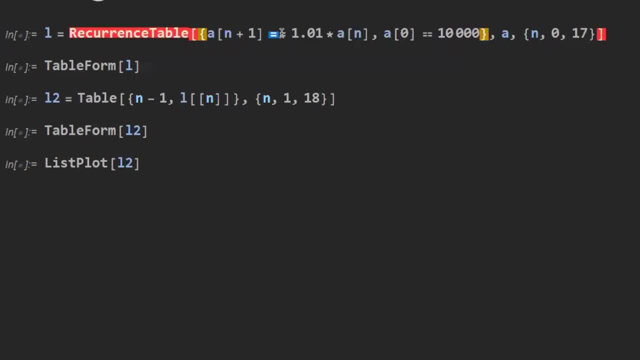 You're going to say a n plus 1.. And it has to be a double equal. Double equal, 1.01 times a n. This is the formula. This one here is the formula I have here Now. you also have to give it the initial conditions. 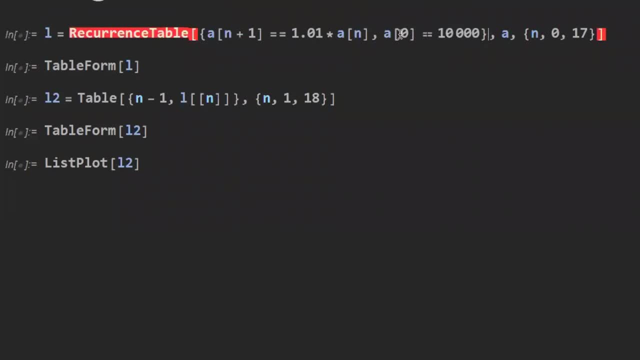 So this is the a0, equal to 10,000.. This in curly braces that you see here. this is where you're going to put your difference equation, here, This one, The initial condition. Put it in between curly braces. This a is the name of your sequence. 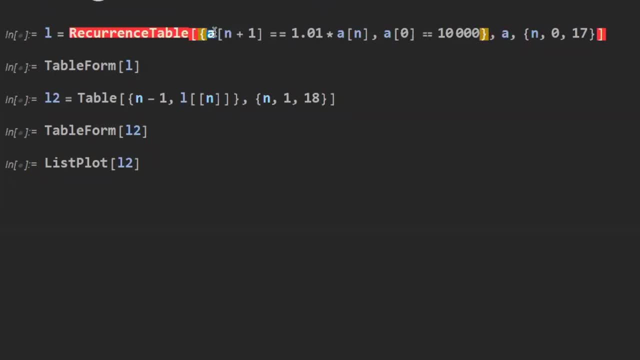 So in this case the name of our sequence is a, So we call it a, And then this open and curly braces that is at the end is telling me here how many values of n I want. So I want to start at 0n, which is the index here. 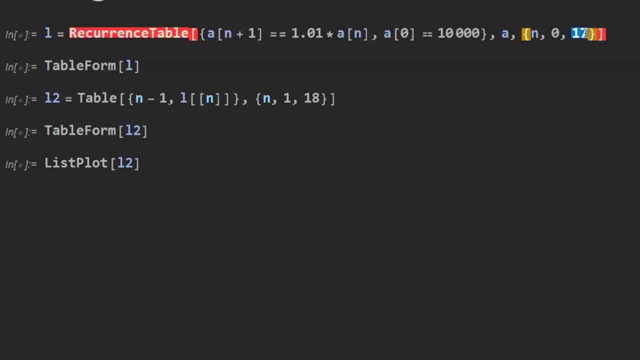 It's going to start at 0 and go all the way up to 17.. I can put here 5 or 10 or 20 or whatever, So let's press enter here and see what happens. So what this is going to give me. it's going to give me the values of that sequence, which. 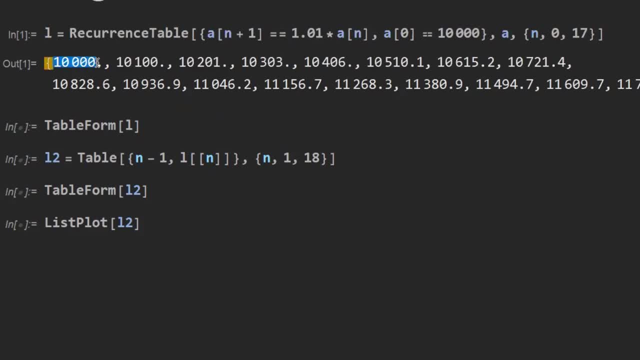 in this case is the savings certificate here. So this is the initial value: 10,000,, 2,100, and so on. It gives me this list. If you change this number here, it will change the number of elements that you're going to. 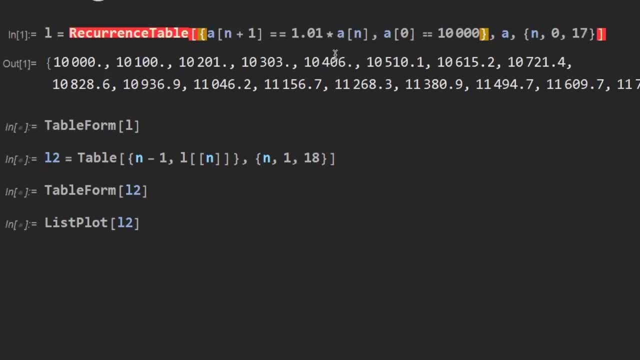 get as an answer here. Now, if you watch the video tutorial for this, It's going to give you the number of elements that you're going to get as an answer here. So if you watch the video tutorial for Mathematica, you know that whenever you have something, 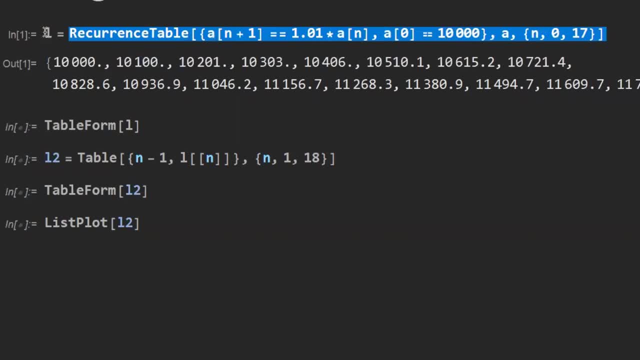 like this and I want to do something else with it. I give it a name, So in this case, I give it the name l, So l equals to. this is going to refer to this list. Now, if you want to see this a little bit better, you can use table form. 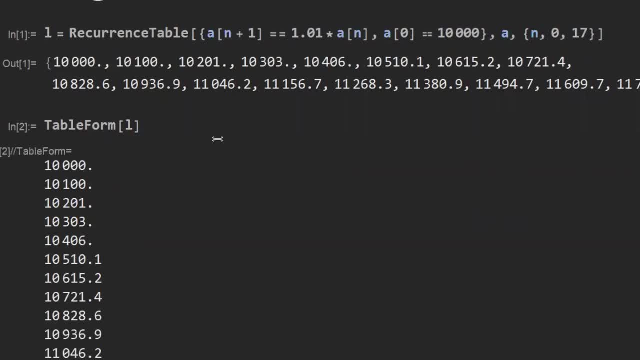 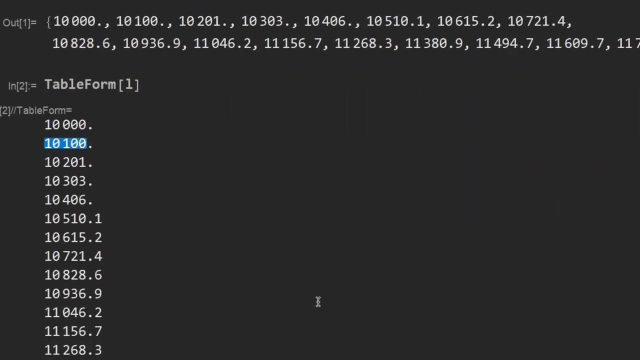 And table form is going to give you this in terms of a column, so you can see this better. So here you have. this is the initial amount, This is at the end of the first month, and so on. Okay, All right. So what is the next thing I'm going to do here? 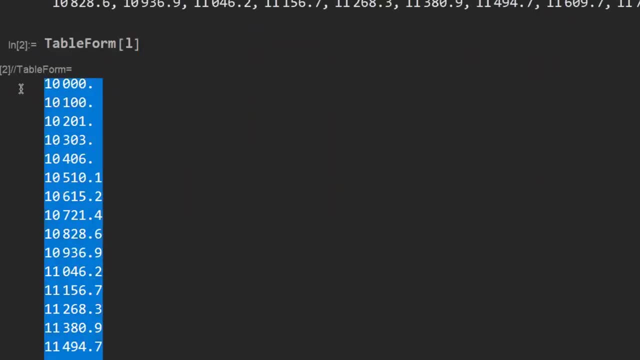 You see, in this table here, I don't have the month here, So I will want to have, for example, 0 is 10,000, 1 is 10,100.. So what I'm doing here is basically make it look better. 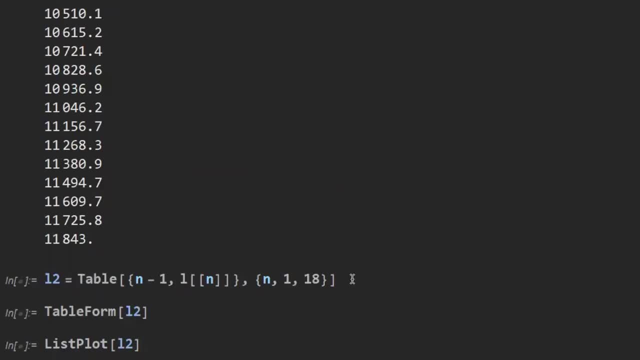 So this here: if you watch the tutorial of Mathematica, this table is going to make a list, A list of two values. The values are going to be 10,000,, 1 is 10,100, and 1 is 10,100.. So what I'm going to do here is basically make it look better. So this here: if you watch the tutorial of Mathematica, this table is going to make a list. So what I'm going to do here is basically make it look better. 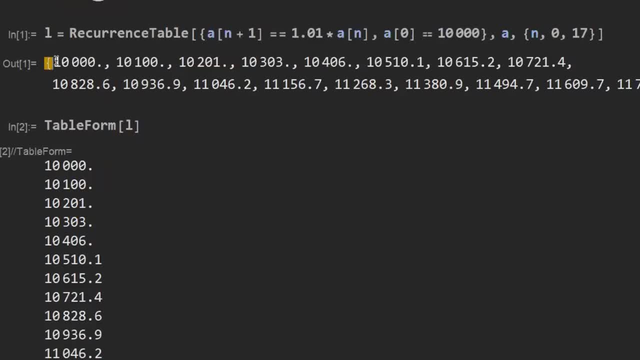 So this here: if you watch the tutorial of Mathematica, this table is going to make a list, And what I'm going to do here is basically make a list of two values, So the value of the end position of the list, L, so L1, L2, L3 and so on in Mathematica. 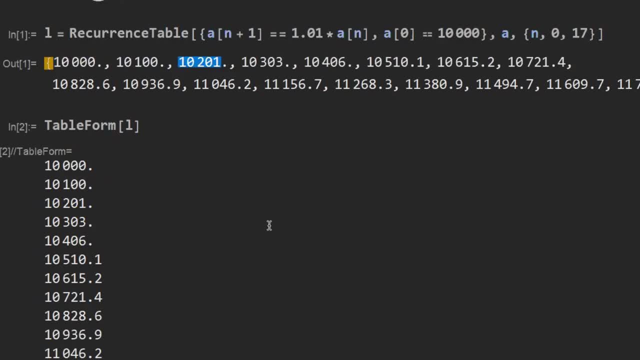 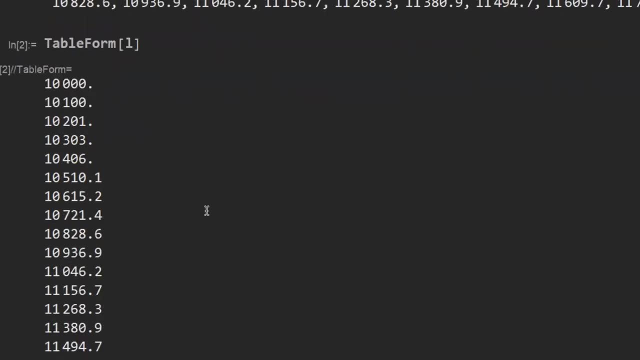 lists are labeled 1,2,3.. So they don't start at 0.. Position 0,, position 1: like you do in computer science, you start at 1.. With list, And I'm going to put the N minus 1 here. 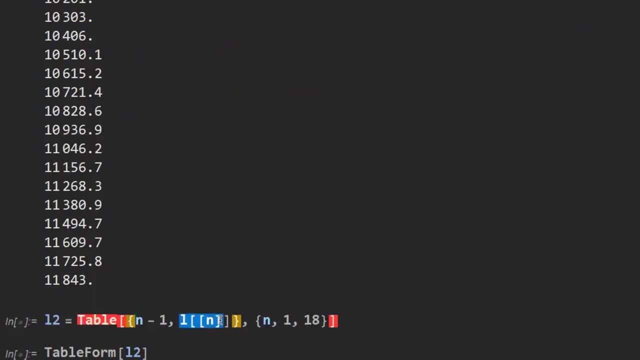 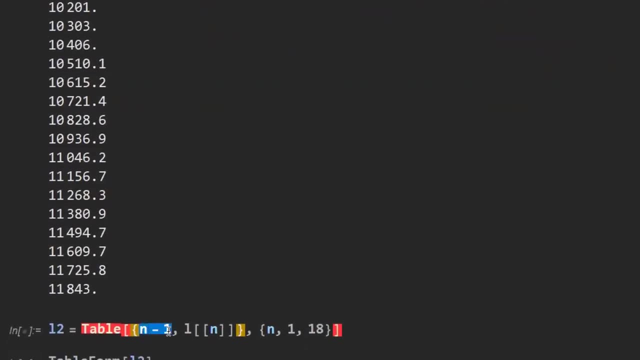 The N minus 1 is basically giving me. so, if it's L1,, which is this, and this is this, and this 10,000. L1 is the initial amount, which is 1 minus 1, which is 0.. So 0, L1,, 1, L2, and. 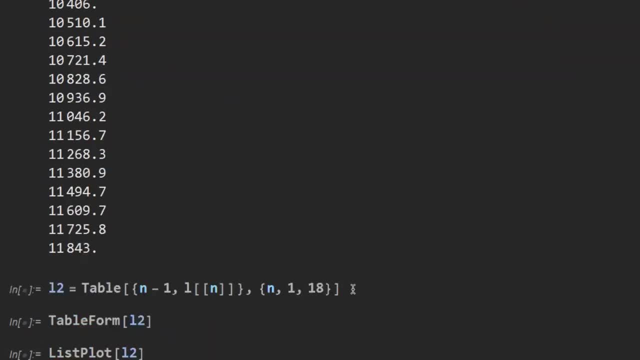 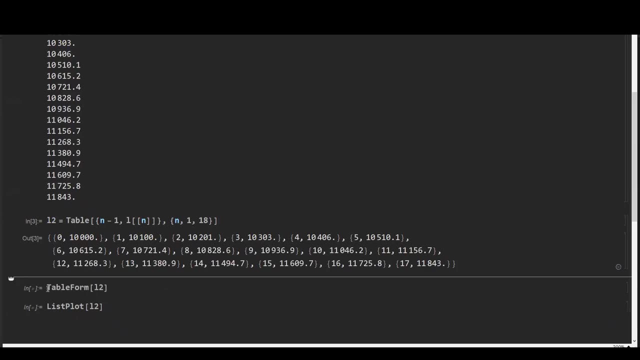 so on. So this here is going to go from 1 to 18 to make sure that we have here all of this. So I'm going to do this. So it's going to give me the pair 0, 10,000.. And if I use, 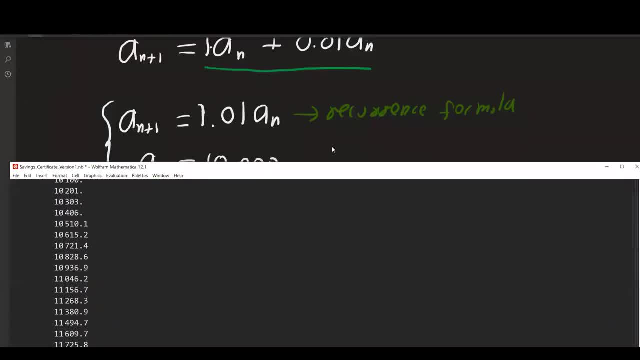 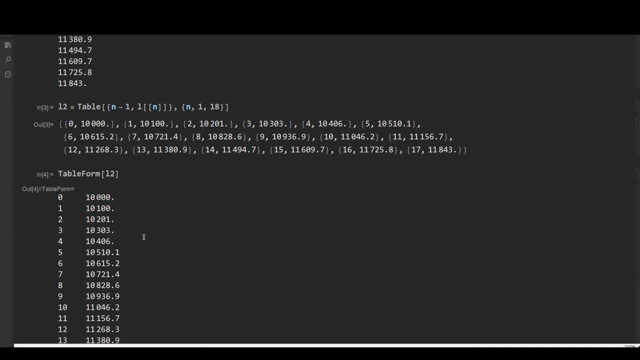 again the table form to make it look like this one, like the one that is here, all of this, then it's going to give me that display here. So 0,, 10,000, and so on. So if you want, 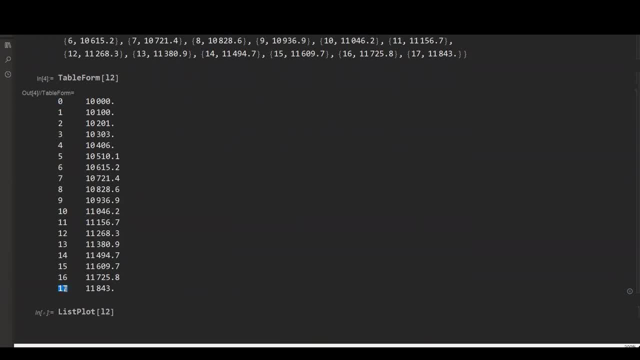 to know what happens in the 17th month of that saving certificate. it's going to give you this much money at the end of the 17th month. So list plot, this is another way to visualize things in mathematics. So when you have list plot, you have a list here that I call L2, which is all of these: 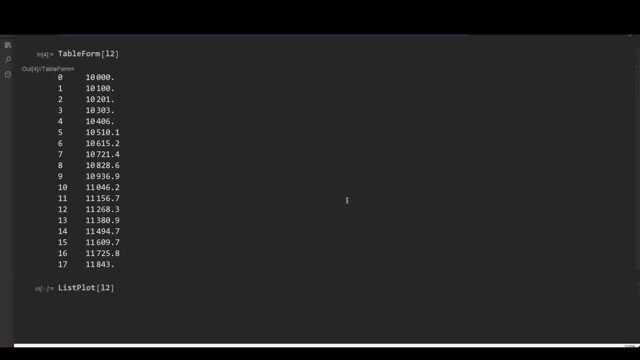 elements in that list of the saving certificate, List plot. what it's going to do? it's going to give me a graphical representation of how that saving certificate is growing. So list plot, or whatever that list is called- In this case I call it L2 because that's what is. 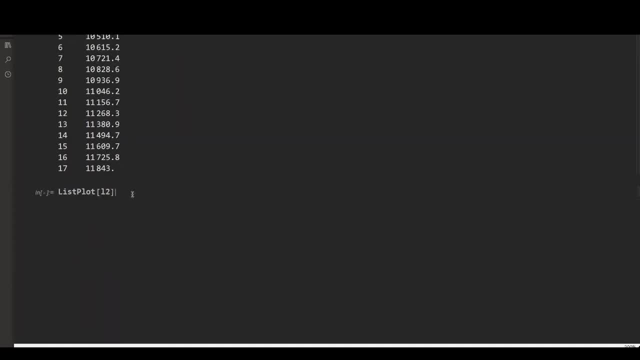 here. This is the L2.. So if I press enter here it's going to give me a list. So we can see here, If we start with $10,000, and at 1% this is going to be increasing here the amount. 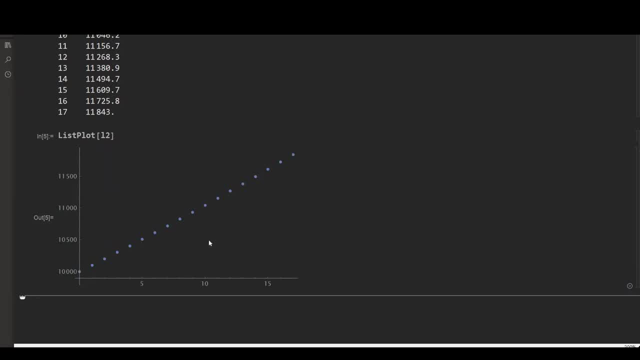 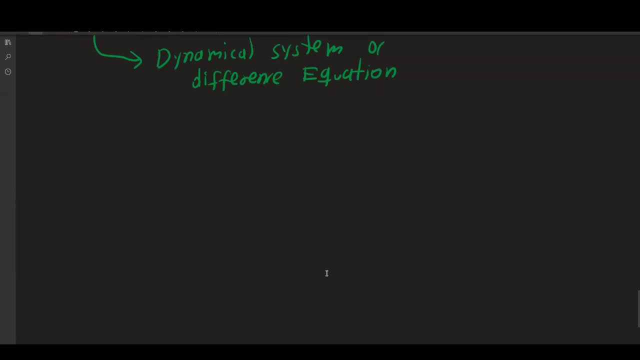 of money in that saving certificate, All right, So let me go back here to OneNote, and I'm going to continue with another example. So let's look at a similar example. but now let's change things a little bit, So let me. 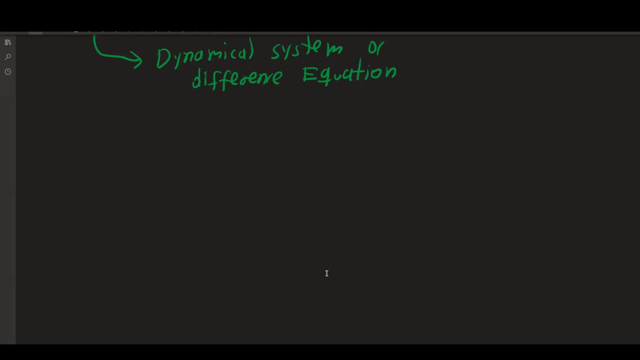 look at this example here And this is going to be that. All right, So this is a continuation with the previous example. Okay, So we're going to modify the previous example as same as in the previous example. Okay, So the same thing: $10,000 initial investment in the saving certificate, 1% of interest. 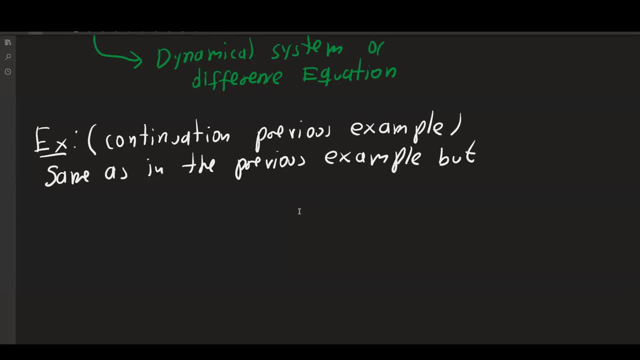 but in this case. but we withdraw $600.. Okay, All right, So let's try to solve the same problem, but now we're going to withdraw from the account every month $600.. So we're going to do a couple of things. The first thing is find delta of an, which is the 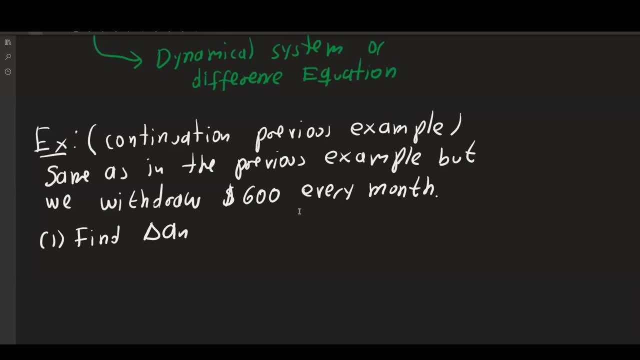 change that happens from present to future. This is in terms of an, in terms of the present, So that's an, And the second part will be find an plus one in terms of an. Okay, All right. Okay, All right. 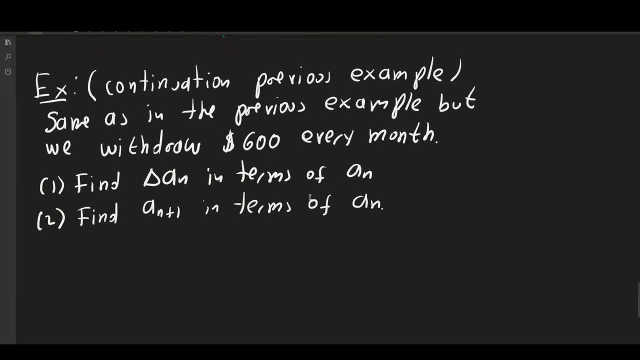 Okay, So let's look at the solution here. All right, So let's draw a picture again of what we have here. Okay, So here we have an. That's the present, And then we have the future, which is an plus. 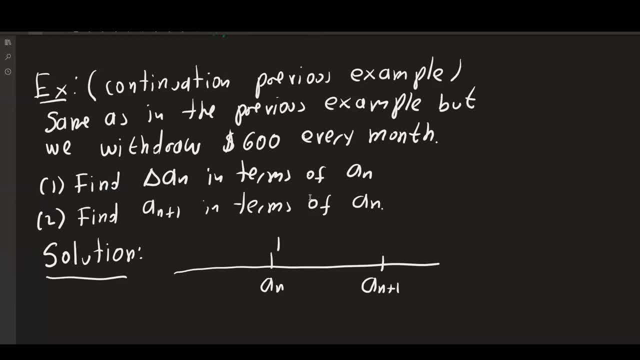 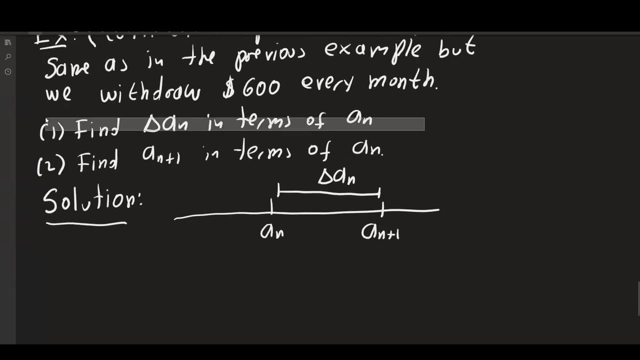 one. Okay, Okay, Okay, Okay, Okay, Okay, Okay. I see the change, which is what happens in that month. So, from the change that happens from present to future. Now the first part of the problem is asking me to find an, the 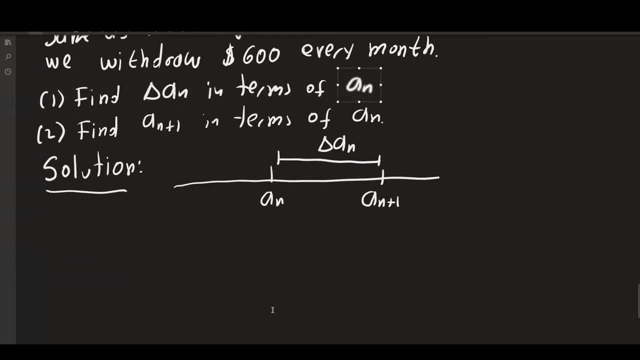 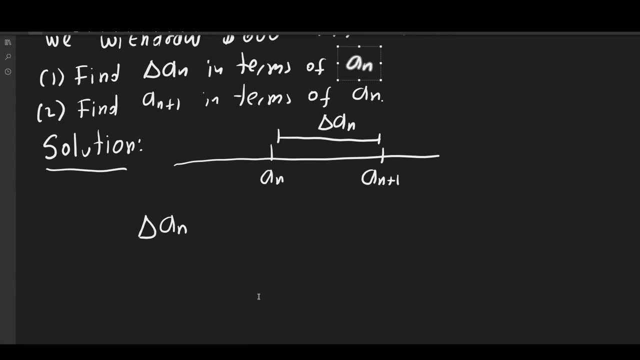 delta of an in terms of an. So let's try to do that. So this is, Let's write down this, So this is the change, All right. Now what happens in this month? Two things happen, right, So very good. 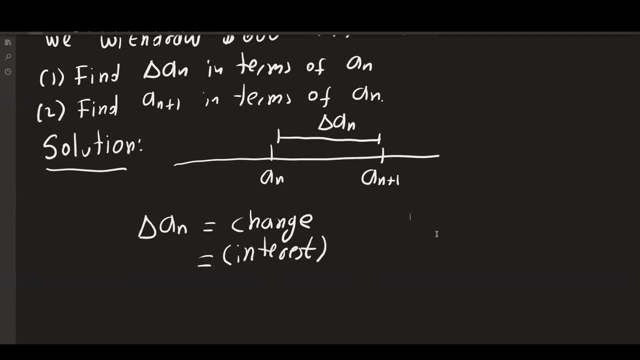 So we have the interest and then minus the withdraw. So that is what happens, or the change that is happening there. Now this interest is an interest of 1%, So this is 1% of AN And here the withdraw is a withdraw that always is constant. 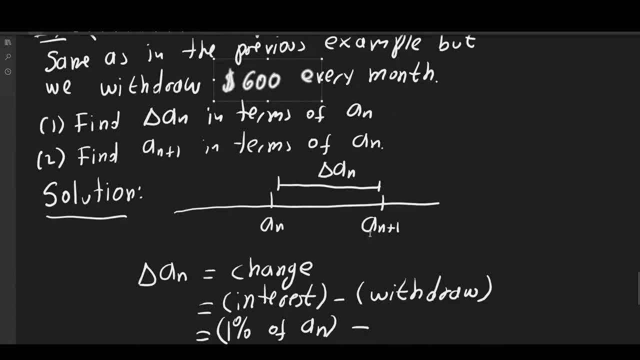 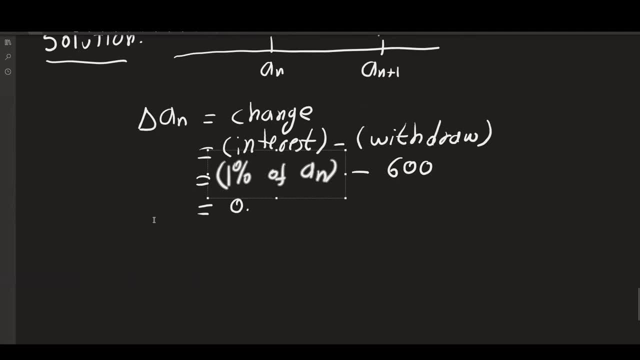 That withdraw is always $600.. So we have this minus $600. So 0.01 AN minus 600.. So that's going to give us the formula For delta of AN. So that's the first part we needed to do. 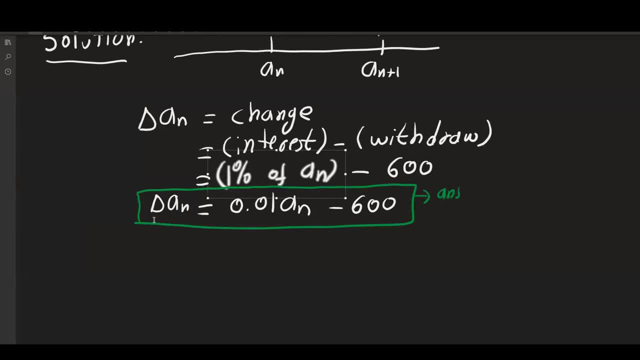 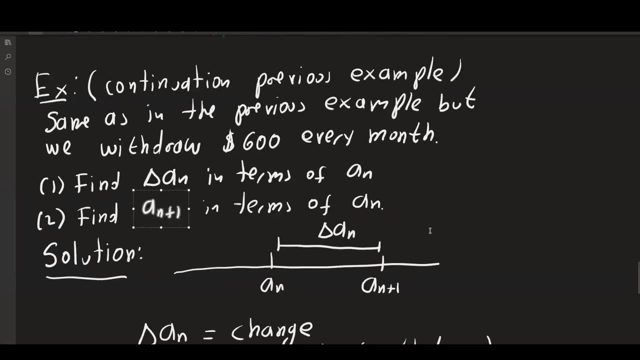 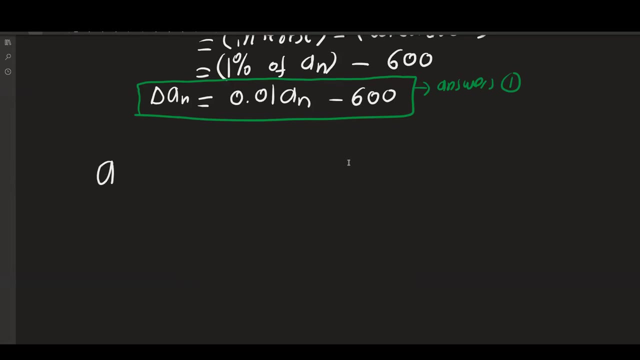 So this answer is number one. So let's try now to find AN plus 1 in terms of AN. So it's always the same formula. So the formula is- because we are taking this type of paradigm- is future value, which is AN plus 1.. 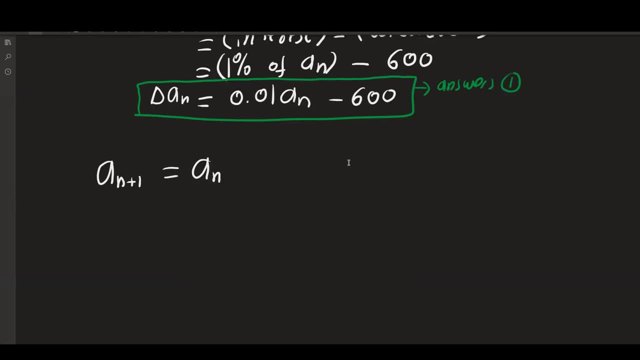 Is it? It's equal to AN, which is the present value plus delta of AN, which is the same, the change. So future value equals the present plus the change. So then we will have our formula. So it's going to be: AN plus 1 equals to AN plus. 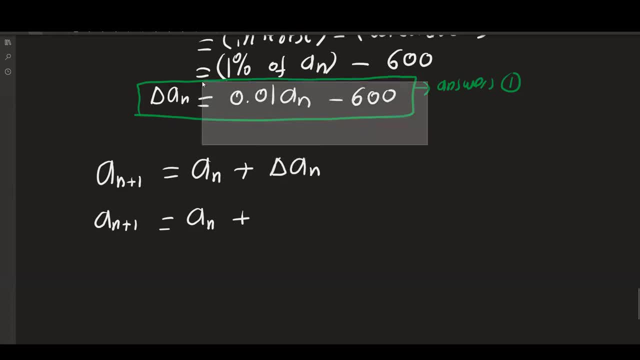 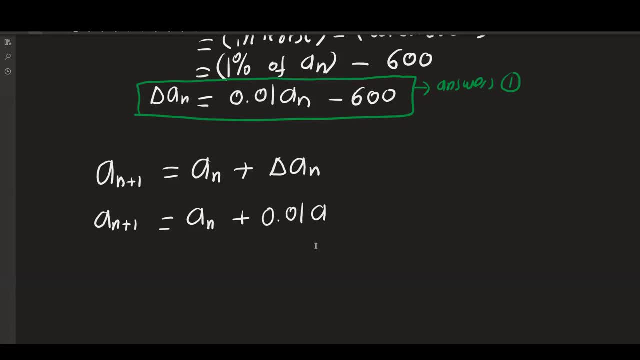 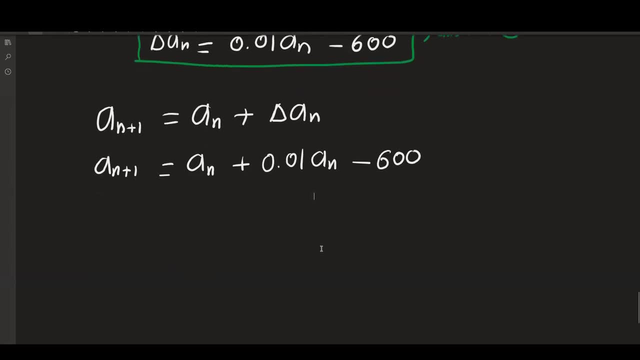 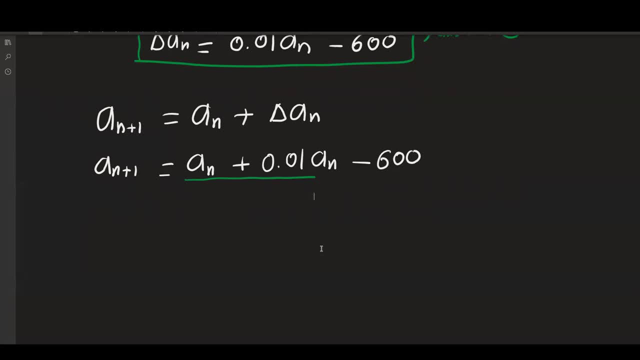 So one more thing here is: you take these two things and you put them together, So then we have the AN plus 1 is equal to just add them. So this is 1.AN 0.01.. AN minus 600.. There Let's complete our difference equation. So our difference. 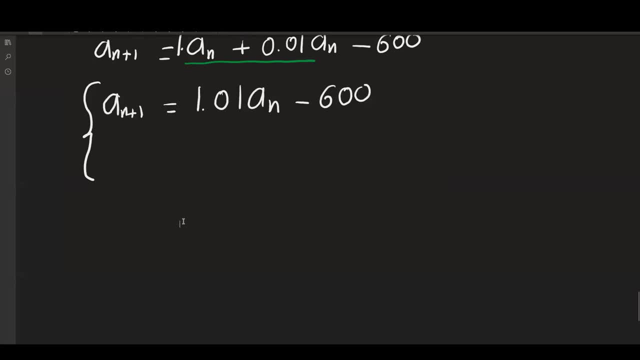 equation will usually have some recurrence relation and we will have to have some initial condition. So the same example as before, but we just we're drawing $600 from the account, which is what this minus 600 here means. Alright, let's look at what happens with this type of situation. So now we are. 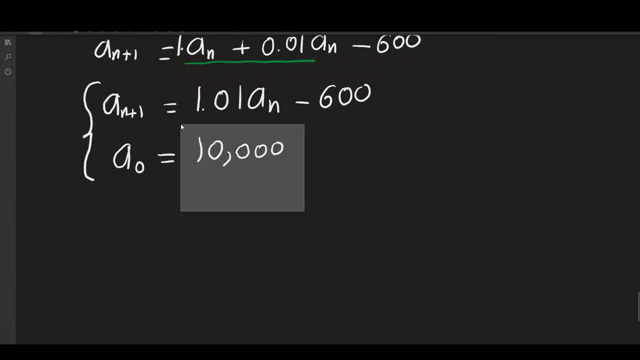 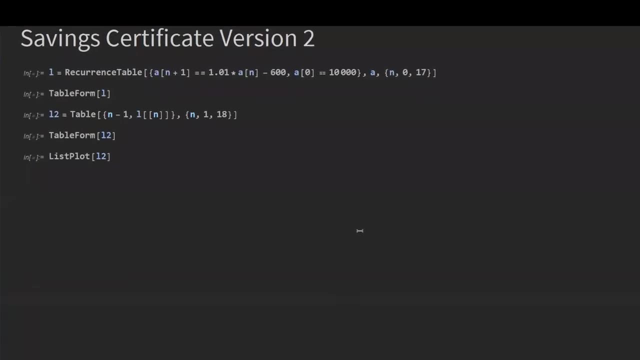 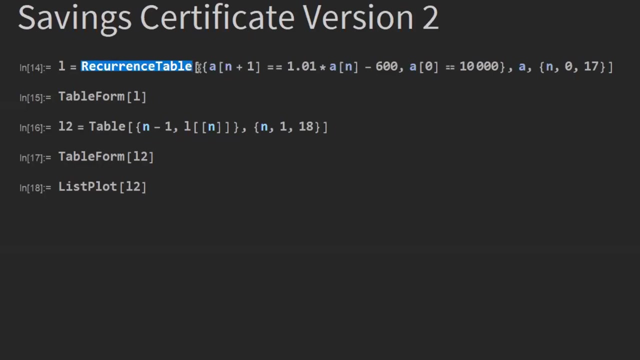 starting with the same thing: ten thousand dollars saving certificate and we have one percent, but now we are withdrawing six hundred dollars. So let me show you this in Mathematica again. So it's similar to what we did in the other, in the other version. So I again have the recurrence table open. close.